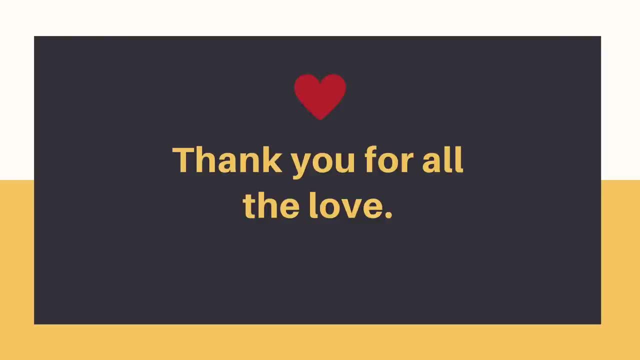 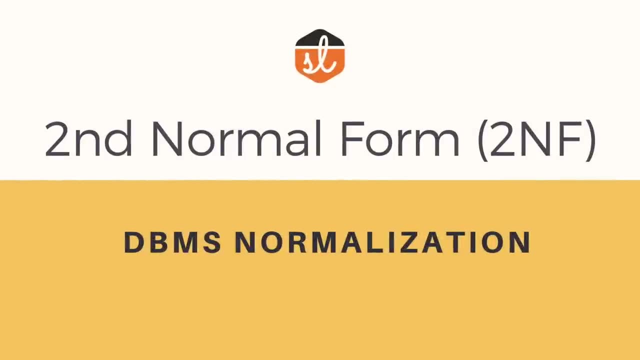 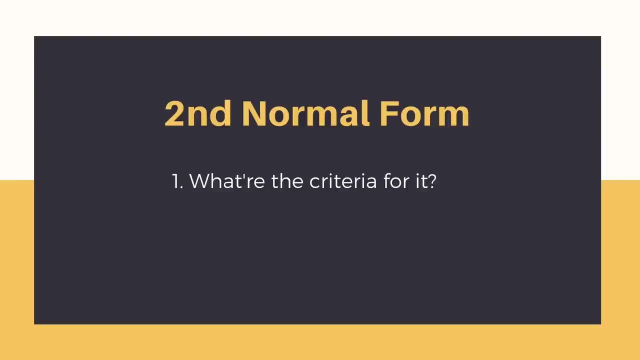 good to know that you guys are equally excited and loving the content. So without any further delay, let's start. In this video we will cover the second normal form of normalization. We will discuss about the criterias required for a table to be in second normal form and why second normal. 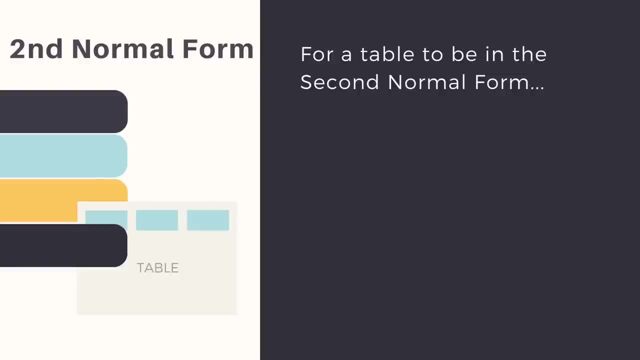 form is so important. For a table to be in second normal form, it must satisfy two conditions. First one: the table should be in the first normal form and the second one: there should be no partial dependency in the table. We have already covered the first normal form. 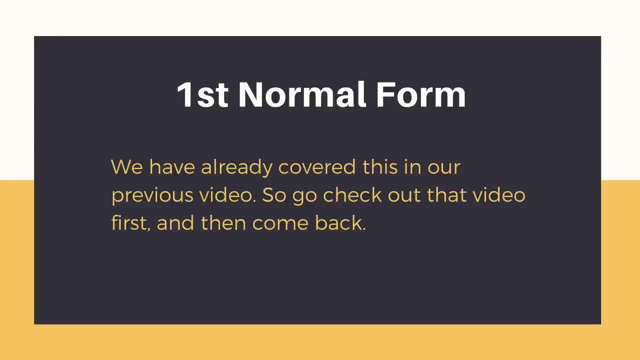 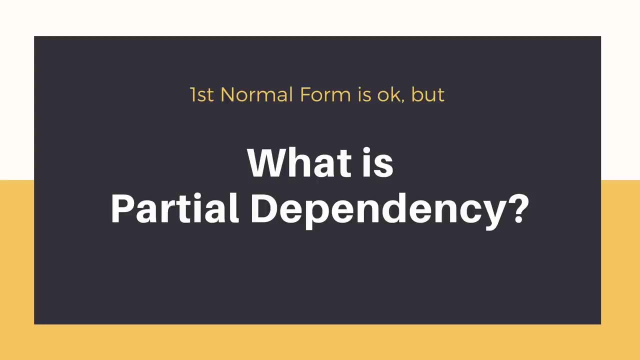 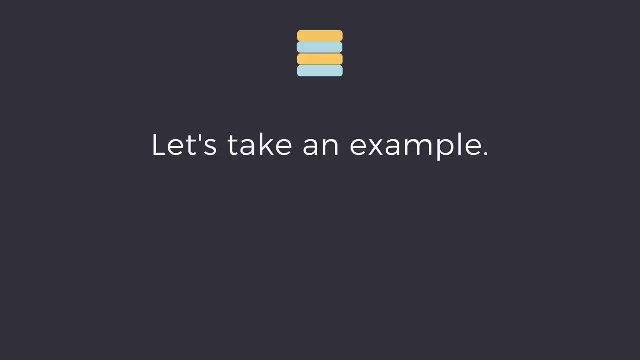 in a previous video. so if you missed that video, we suggest you to go check out that video first. Now the main question is: what is partial dependency? To understand partial dependency, we first need to understand what dependency in a table is. So let's take an example of 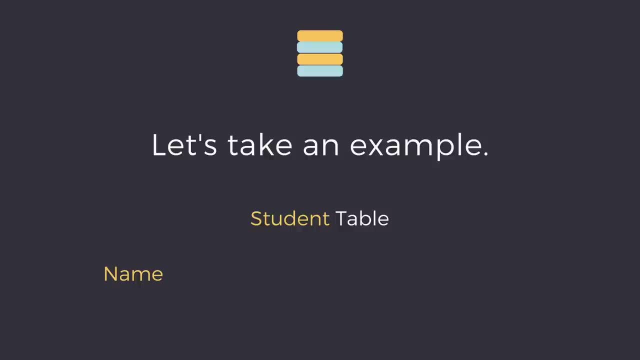 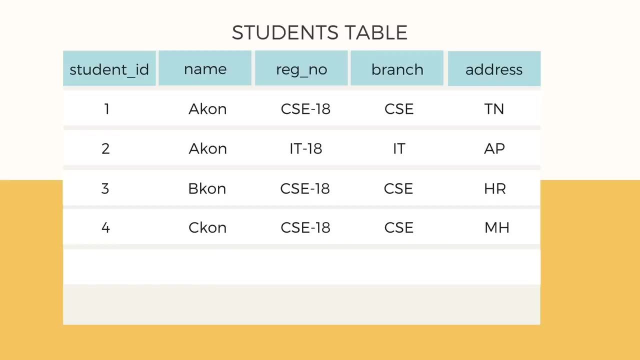 a student table in which we save student's name, student's registration number, student's branch and student's address, etc. In this table, student table has a second normal form. In this table, student's name, student's registration number. 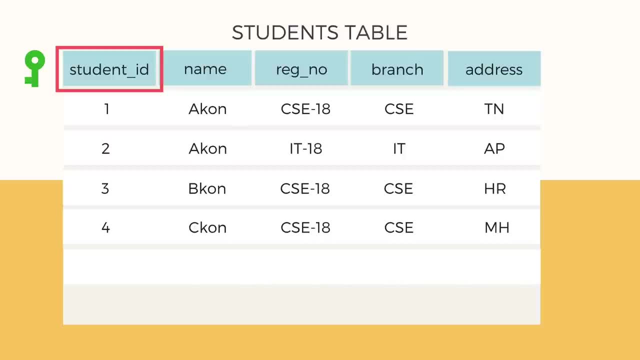 ID is the primary key and is unique for every row. Hence we can use the student ID to fetch any row from this table, even for a case where student names are same. If we know the student ID, we can easily fetch the correct row or column of data. 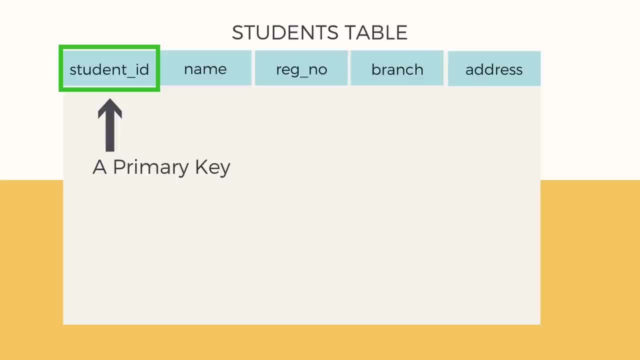 Primary key is nothing but a column, or, at times, a group of columns, which can uniquely identify each row in the table. or, in simple words, all you need is the primary key to fetch any data from the table. For example, I can say: give me the branch name of student with ID 10 and I can get it Similarly if I ask for name. 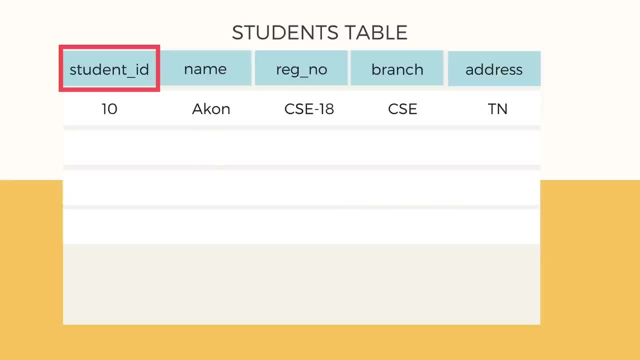 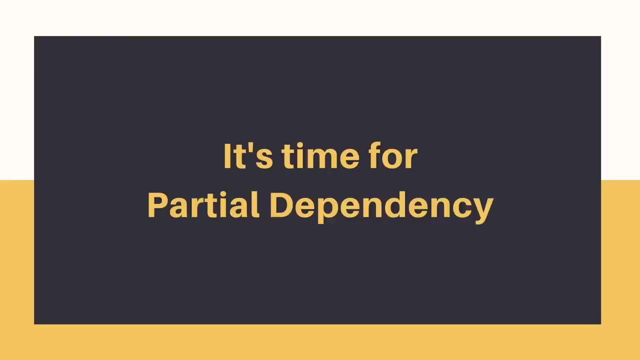 of student ID 10, I will get it. So all I need is student ID and every other column depends on it. This is dependency in table. Now that we know what dependency is, we are in a better state to understand what partial dependency is. So, for a simple table, like student, a single column which is student. 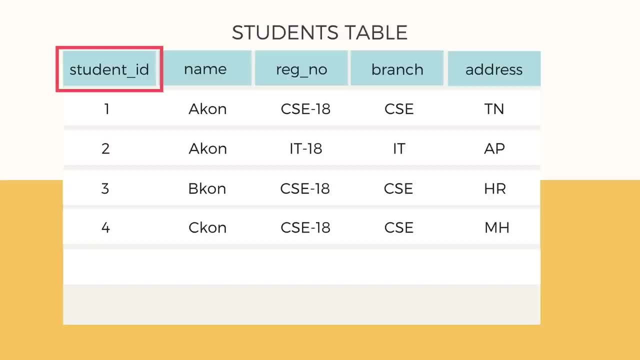 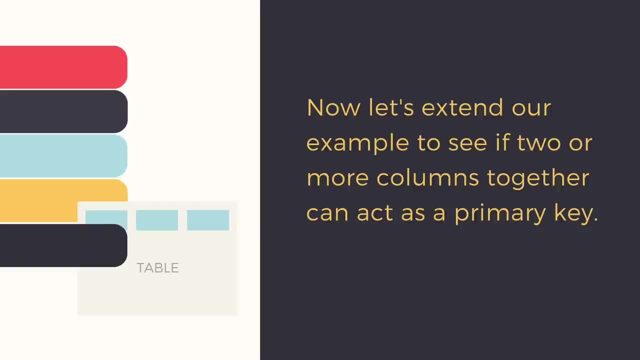 ID can uniquely identify the complete row or all the other columns in a row, But this is not true all the time. Now let's extend our example to see if more than one column together can act as a primary key or not. Let's create another. 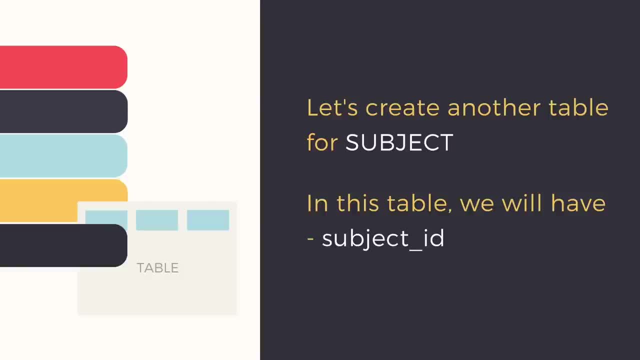 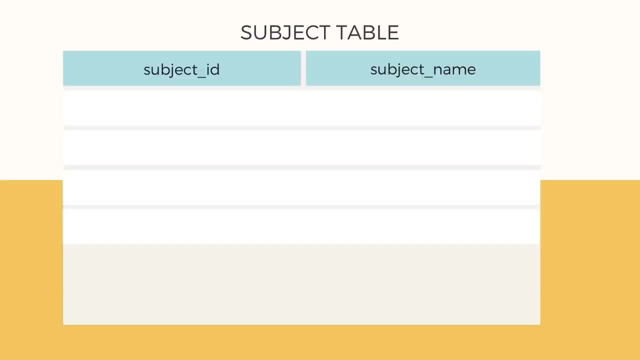 table for survival. In this table we have subject ID, which is the primary key for this table, and the subject name. Again, subject ID can be used to get all the information stored in all the other columns. Unfortunately, there is only one other column in this. 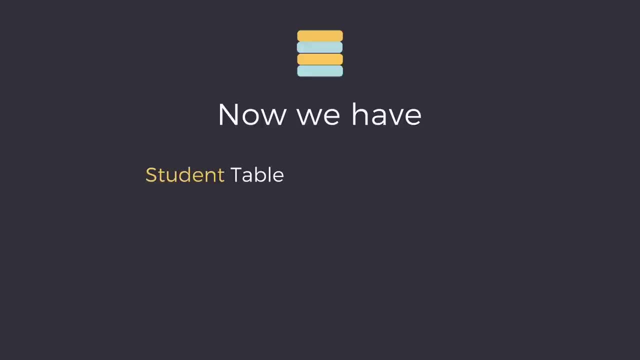 case. Now we have a student table with student information and another table for subjects. During exams, another table score is created to store the marks obtained by every student in the respective subjects. Also, name of the teacher who teaches the subject is saved along with the marks. So 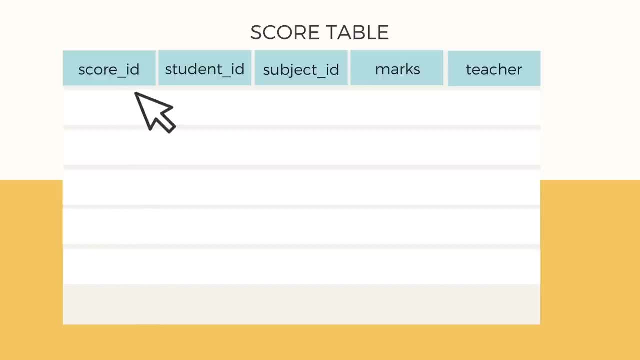 in our score table we will have columns, score ID, student ID, subject, ID marks and teacher name. Let's add some data to this table. As you can see, in the score table we are saving student ID to know which students marks are these Subject. 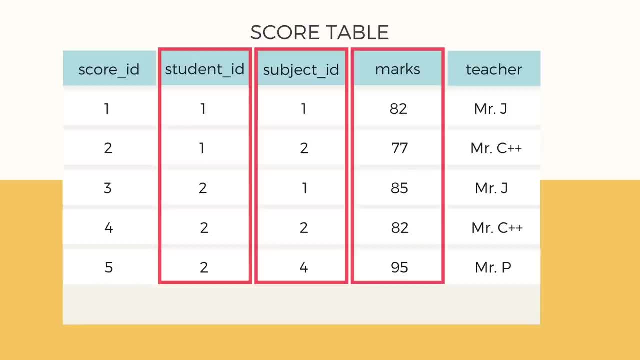 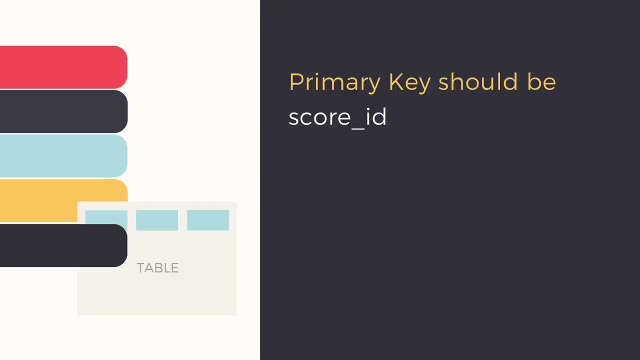 ID to know for which subject the marks are and the marks and the teacher name. In this table we can say that the primary key is score ID, but student ID and subject ID together forms a more meaningful primary key for this table and we can fetch all the information using it. You would ask how? See if I ask. 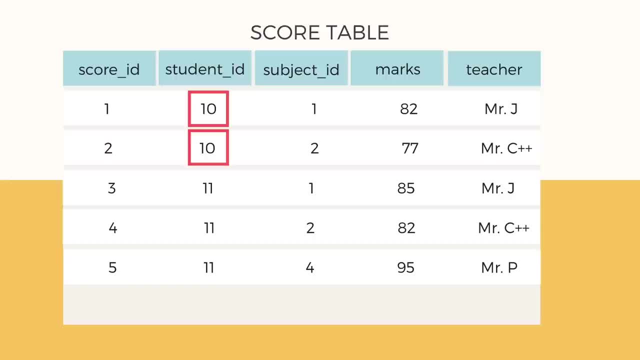 you to get me marks of student with student ID 10. can you get it from this table? No, Because you don't know for which subject and if I give you a subject ID, you don't know for which student. Hence we need student ID and subject ID together to 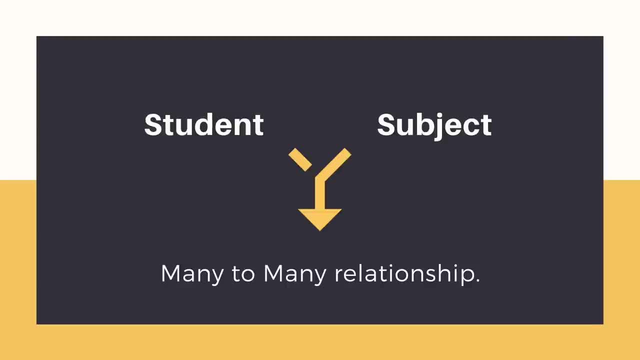 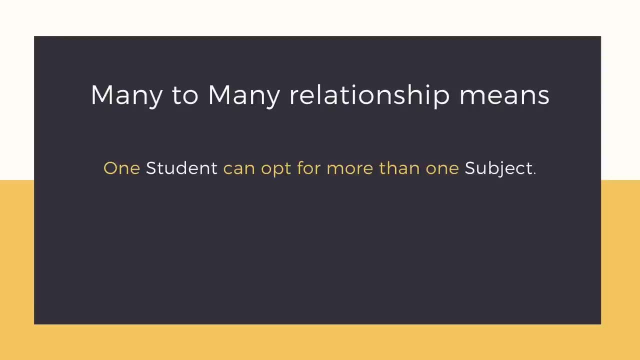 uniquely identify any row of data, because we have a many-to-many relationship here. When I say that we have a many-to-many relationship here, I mean a student can appear for any number of subjects test. Also, a subject can be opted by any number of students.